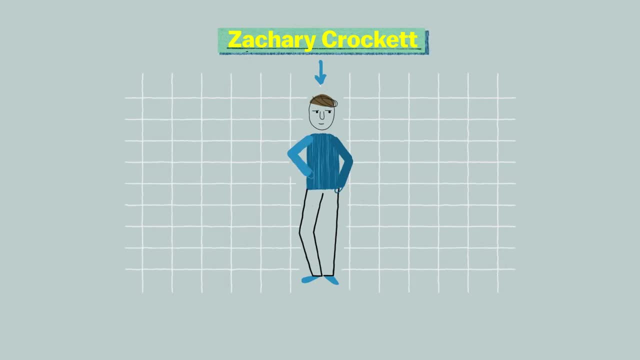 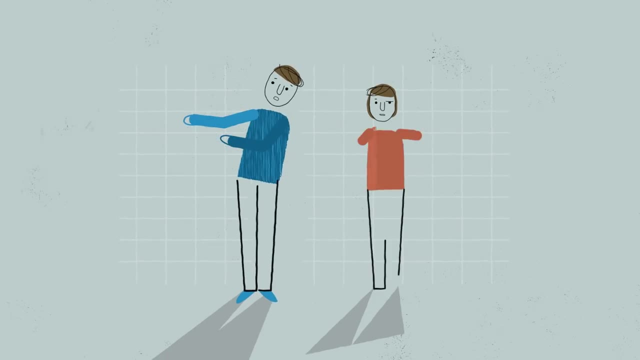 before we dive in, I'm going to introduce you to Zachary Crockett. He first introduced me to the puzzle and I called him up to talk about it. My name is Zachary Crockett. I'm a writer for Priceonomics. Zachary and his girlfriend were stumped by the problem too. We just like. 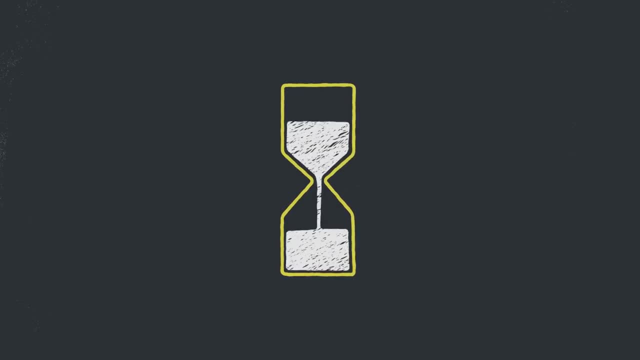 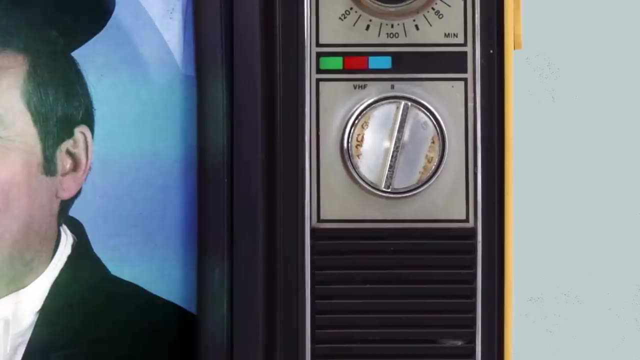 sat there debating the answer to this problem for two hours and I don't think either of us really understood it. The puzzle we were all stumped by is called the Monty Hall problem, named after the host of the game show that made it famous. You see, the problem goes like this: 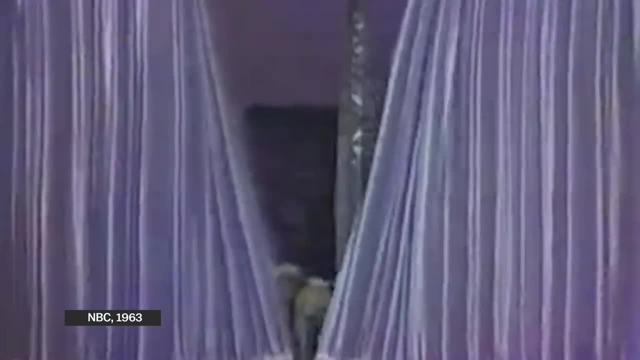 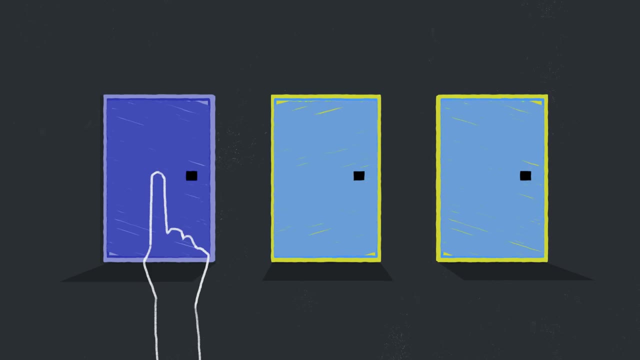 There's a brand new car behind one of three doors. Behind the other two are goats. Say you pick door number one. Monty then shows you the goat behind one of the doors you didn't choose. Say door number three. Now here's the question: You're allowed to change. 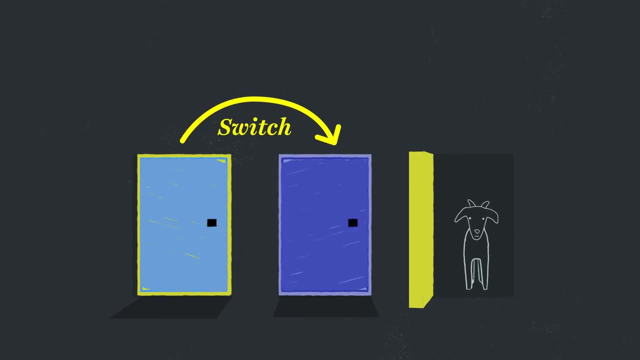 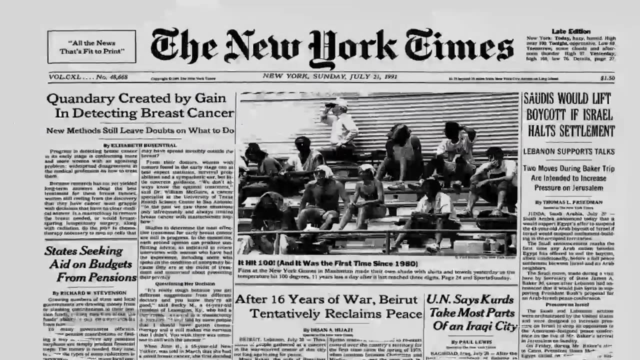 your answer to door two. Do you switch Or do you stick with your original choice? But yeah, I got interested in the Monty Hall problem, did a little research and then I found out there was this whole kind of second angle to the story. 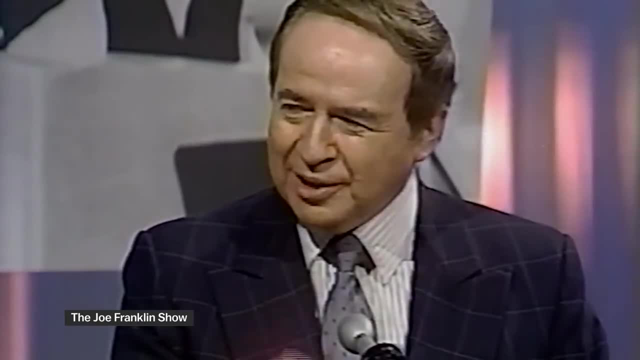 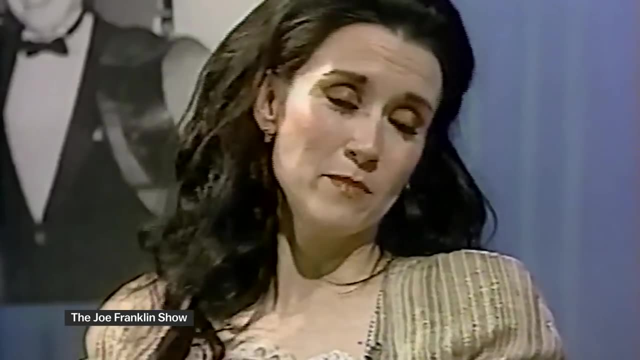 Never met a man who feared you a little bit because he thought you were much brighter than he was. That's Marilyn Vos Savant in 1988, being interviewed by Joe Franklin. Well, yeah, maybe I met a man like year two, maybe a couple hundred like that. 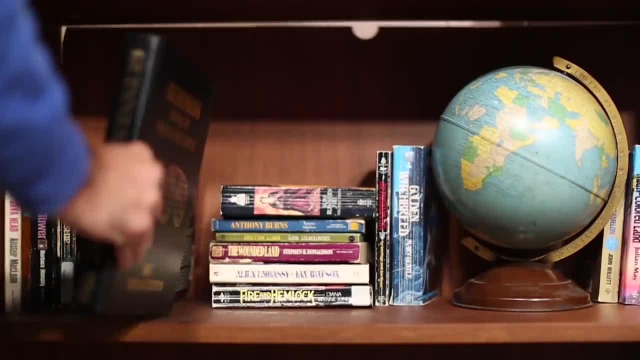 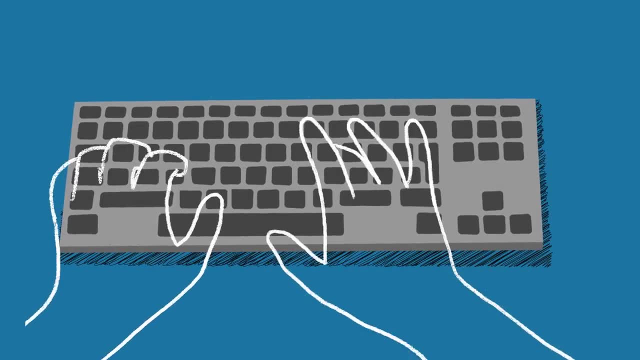 Marilyn is very intelligent. In fact, back when the Guinness World Records actually kept track of this, she was the world's highest IQ. She now writes for Parade magazine and has for the last 20 years. So the premise of the column was, of course, like: here is the person with the world's highest IQ. 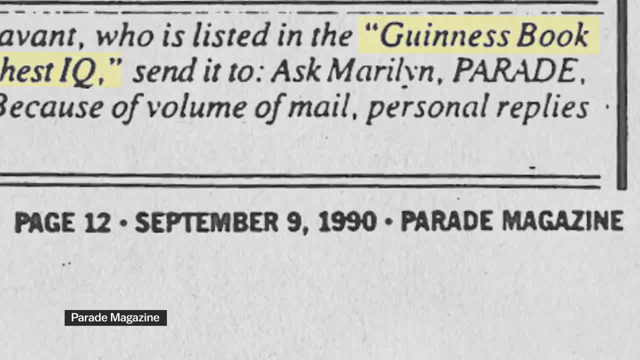 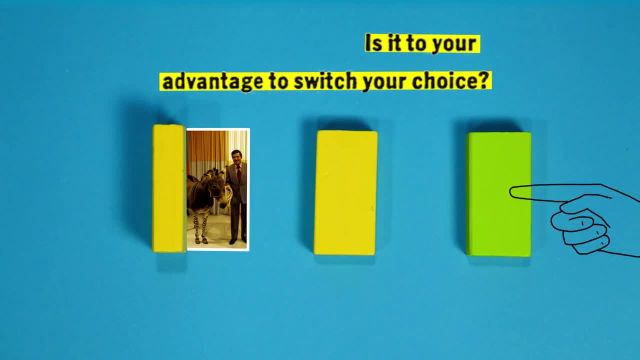 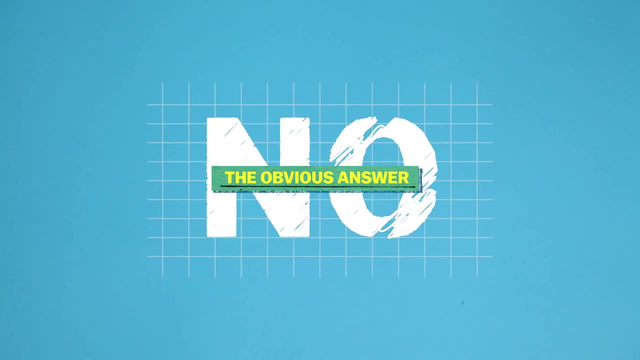 here to answer your challenging math questions. This brings us to September 9th 1990, when a reader submitted to Marilyn the Monty Hall problem. Is it to your advantage to switch your choice of doors? Now, if you're like me, the obvious answer is no. There are two doors, So the chance of getting a 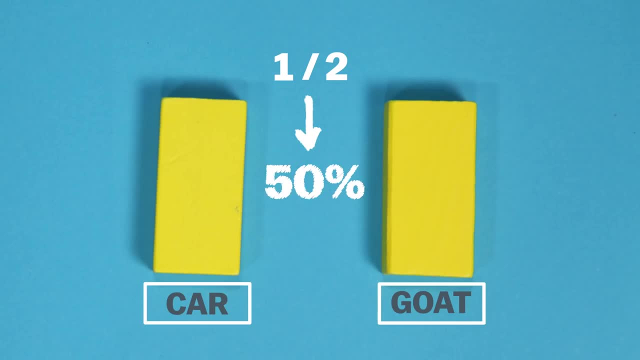 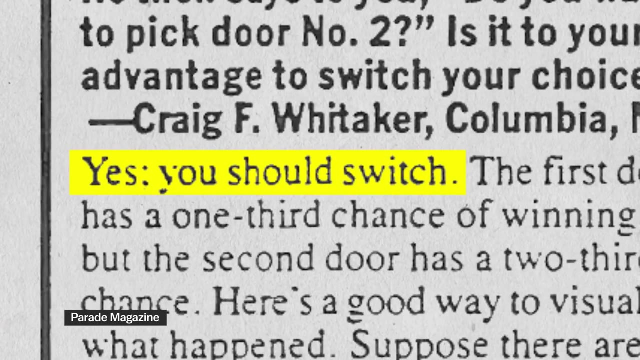 car and not a goat is 50-50.. Bing, bang, boom. But that's the wrong answer And Marilyn knew that. She replied: yes, you should switch, And here's why Here are three doors. There is a goat behind two and a car behind one. 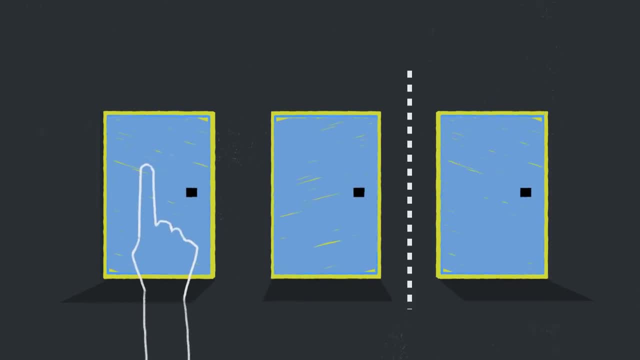 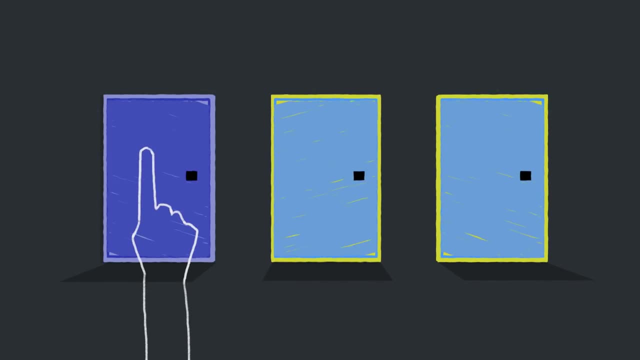 Here is why, In a blind test, you're more likely to pick a goat than a car. In fact, you're two thirds likely. So let's use that as the main scenario. You pick door one. So now Monty Hall, who knows what's behind all the doors, is forced to reveal a goat. 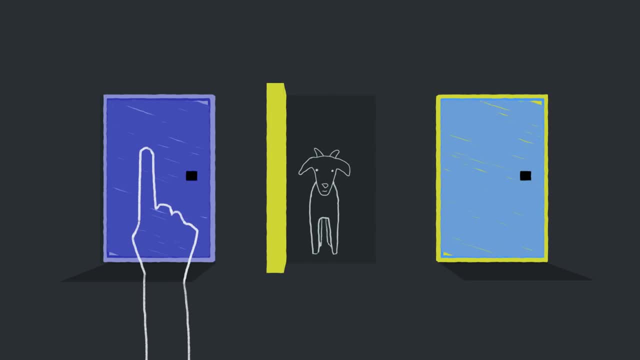 regardless of the door you pick, Since, in the most probable scenario, you've also picked a goat, the only door left is the one with the car. So now Monty Hall asks: would you rather keep the door you've picked or would you switch? 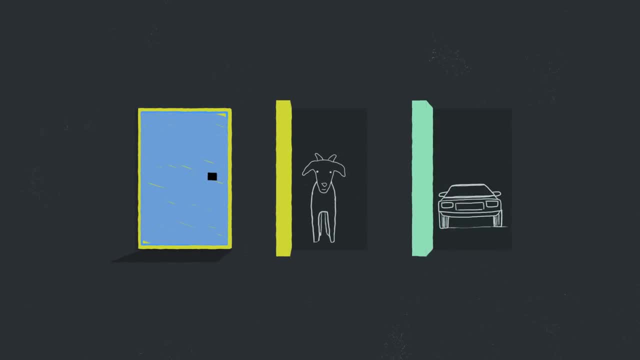 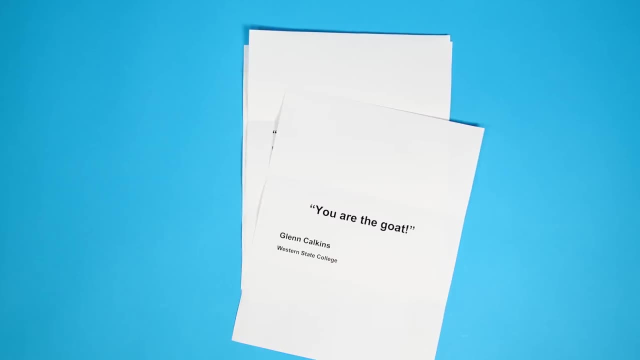 Definitely switch. If you do, you get the car two-thirds of the time", Turns out. when Marilyn correctly answered the Monty Hall problem, she received thousands of letters from across the world telling her she was flat-out wrong. I think part of her was kind of a little bit surprised that she received 10,000 letters. 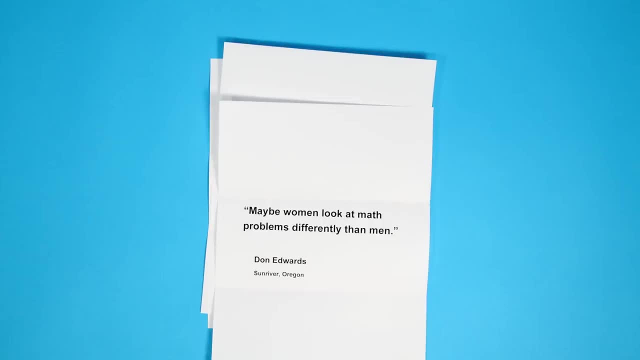 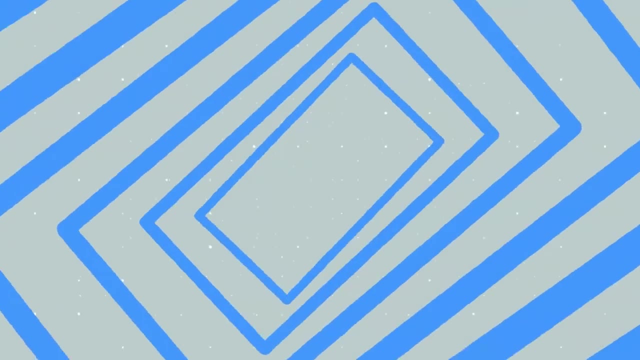 calling her an idiot. There was, without a doubt, a little bit of sexism at play here. Not only was her answer right, it wasn't anything new. The first time the Monty Hall problem was really conceived was in 1975.. 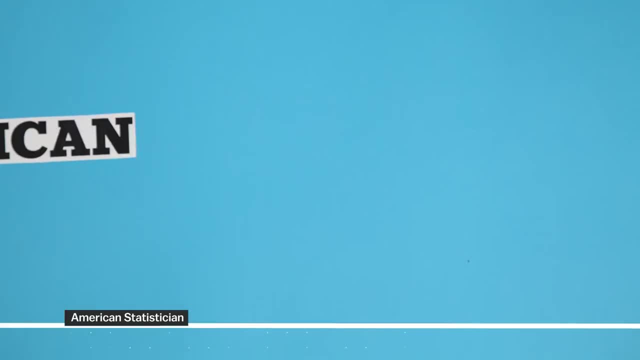 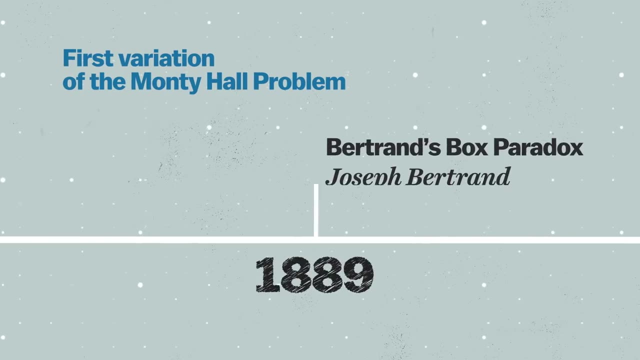 So this guy named Steve Sullivan at Berkeley presented this problem in The American Statistician. He contested that the odds were two out of three and no one argued with him. You know, over the next 15 years multiple other academics reiterated the same problem. 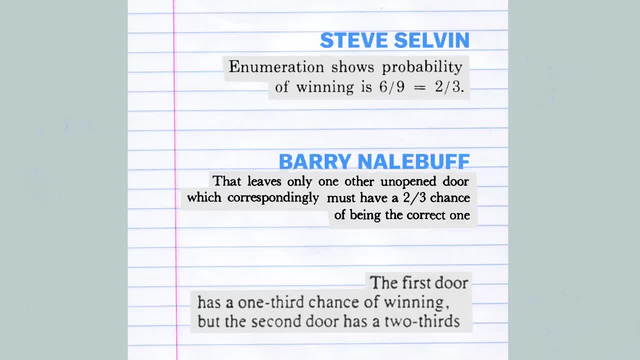 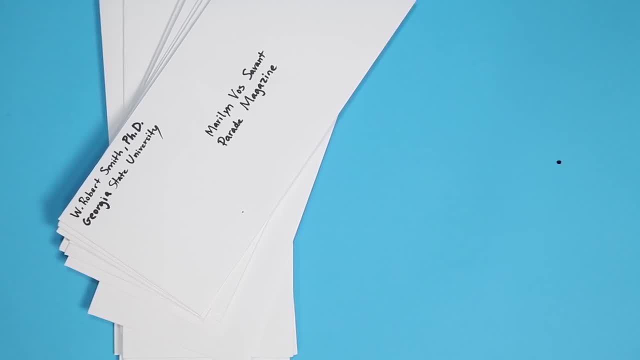 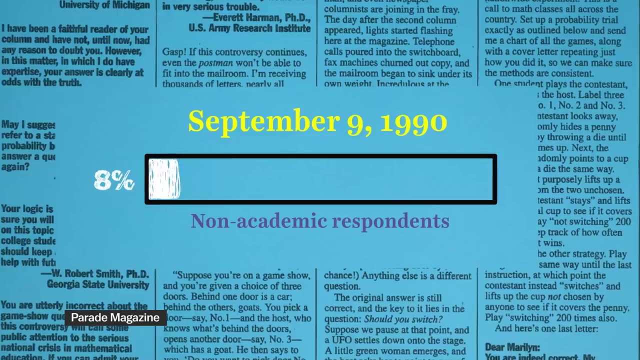 and no one ever told them they were wrong. Then in 1990, Marilyn answered the same question correctly and people went bananas. Marilyn ended up tallying up what percentage of the 10,000 responses claimed she was wrong. Only 8% of readers actually agreed with her. 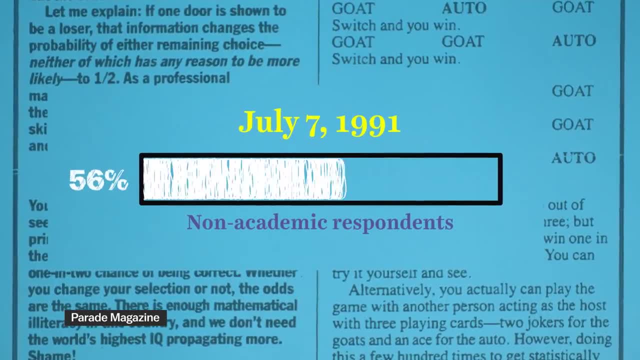 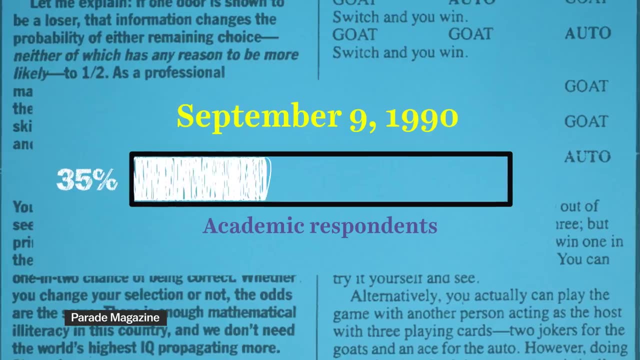 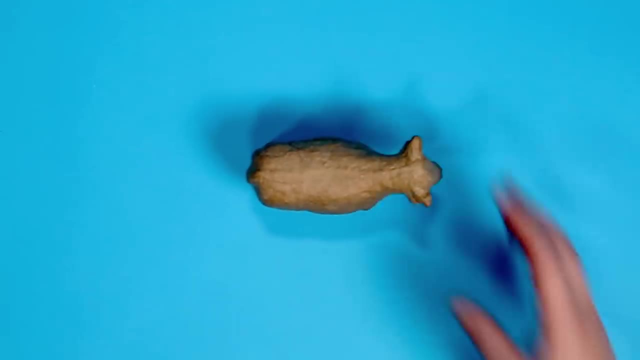 And after subsequent columns she was able to raise that to only 56%, And among academics It was 35%. among academics initially supporting it, Around 70% of academics ultimately decided to agree with her. The only way she managed to get people on her side was by asking them to do the math. 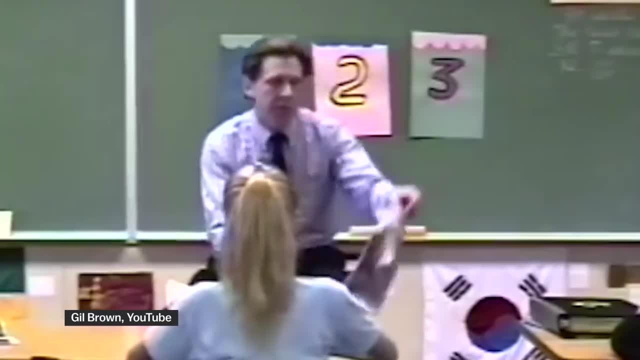 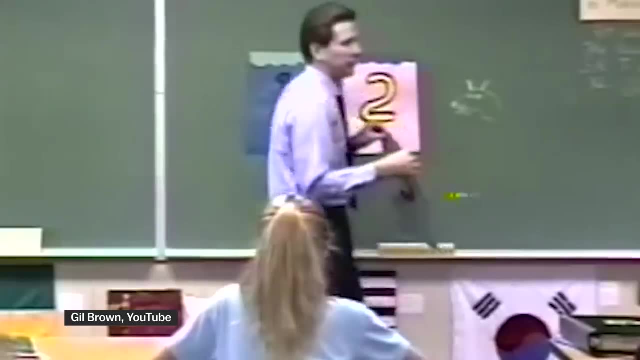 And she did. She even asked them to do the experiment themselves. Elementary, middle school and high school teachers from all over the country wrote in, astounded that their students were able to prove her right. It's easy now to do a simple Google search of this little sucker of a problem and get.